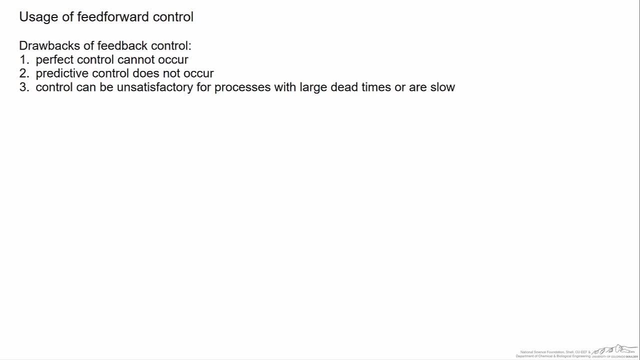 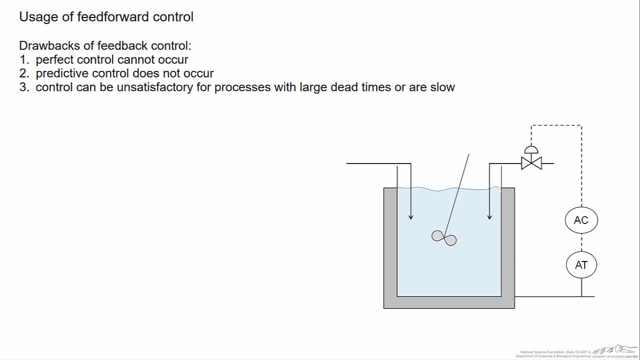 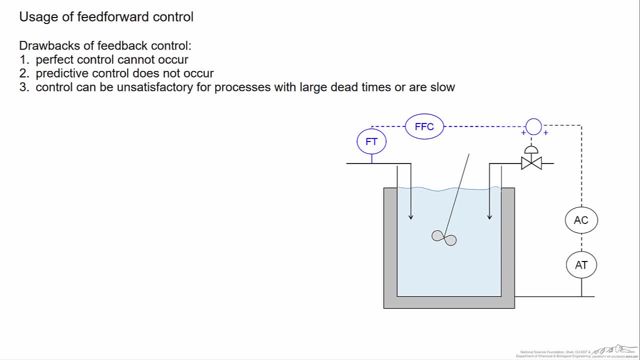 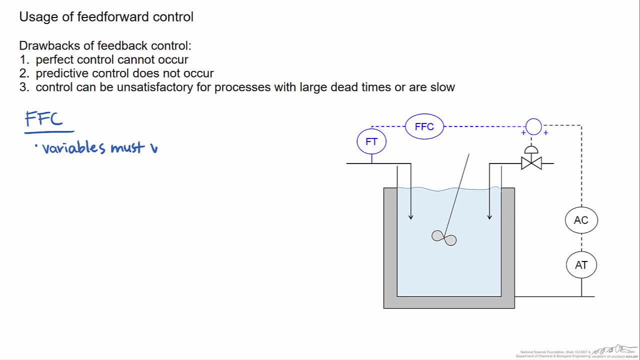 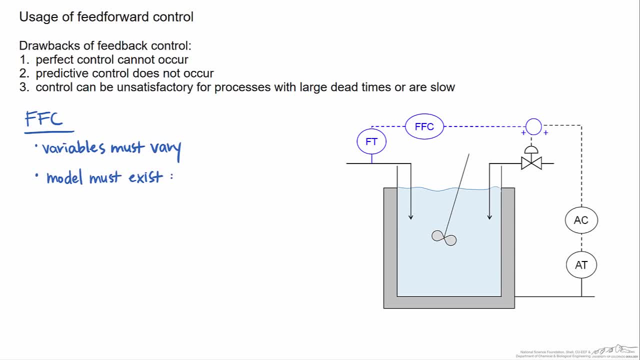 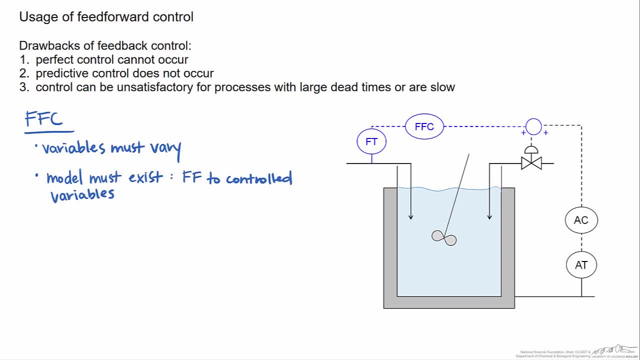 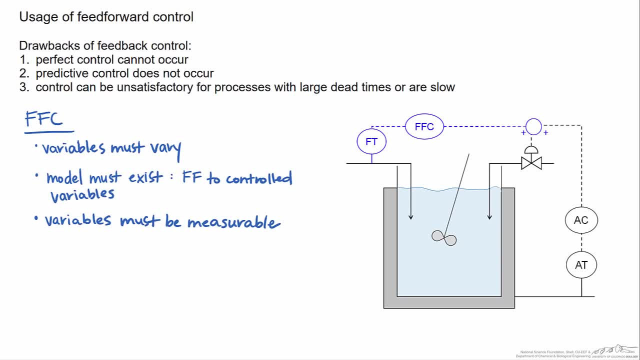 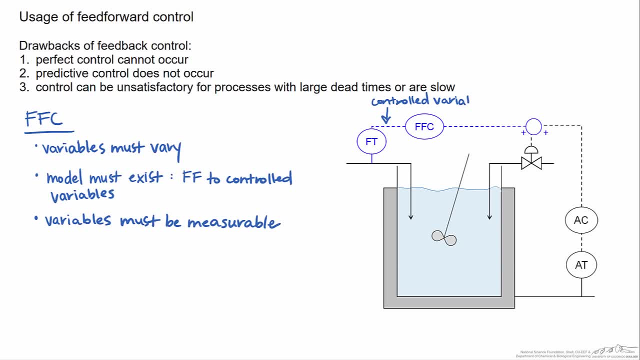 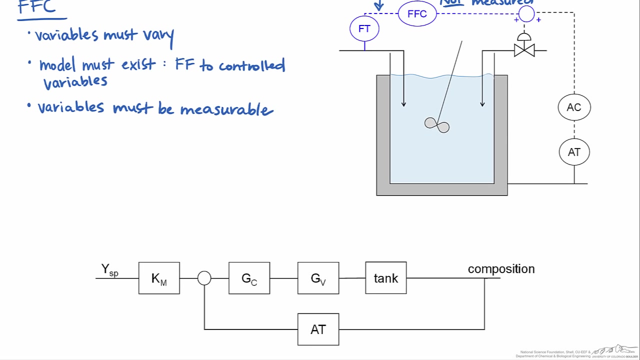 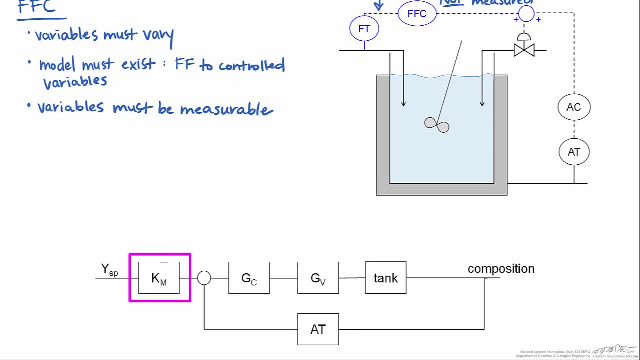 transmitter, we'd have a set point with an appropriate gain. it would then go to the controller, the valve, the process, which here is the tank, and then out would come the composition. So therefore, this part has been maintained by this process. However, the question to 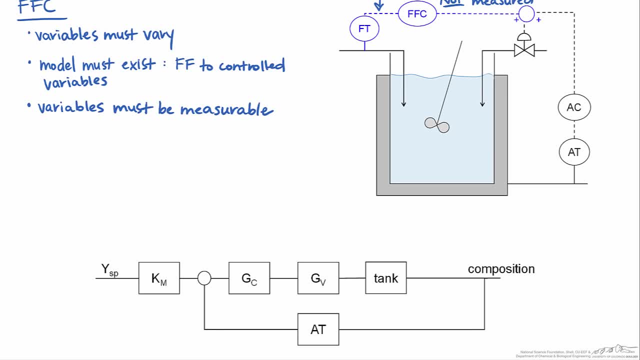 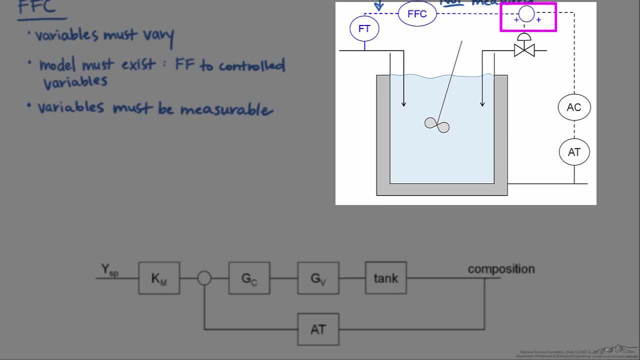 ask ourselves is: how does the feed forward controller fit in? And the way we can gain some insight on this is kind of looking at the diagram. What we notice here is that, right before the valve, instead of it receiving one controller signal, it now receives two. 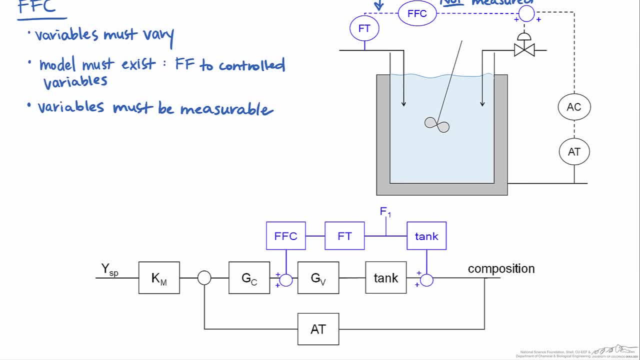 Both sum together and the other one is the feed forward controller. The feed forward controller gets a signal from the flow transmitter, which means the fact that the flow transmitter has to take into account the measuring of the flow rate of that stream, which we'll 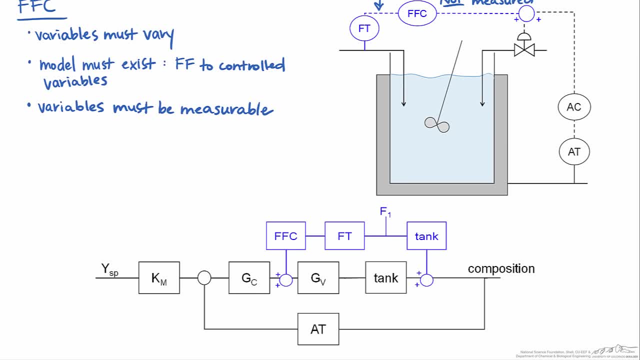 call here F1.. By adjusting F1, I am also adjusting the composition. So therefore there is a second tank transfer function here that represents the relationship between F1, the disturbance variable and the composition coming out of the tank. So therefore we have another block. 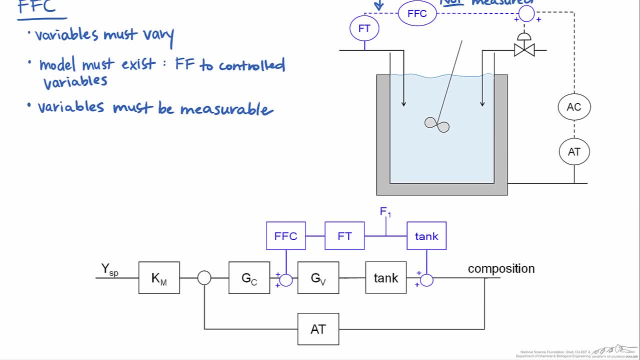 which shows that relationship. So, therefore, the composition here changes because of two things: The change of the flow rate of the first stream and the flow rate of the second stream, which is being manipulated by the valve. This relationship would come out through a material balance. 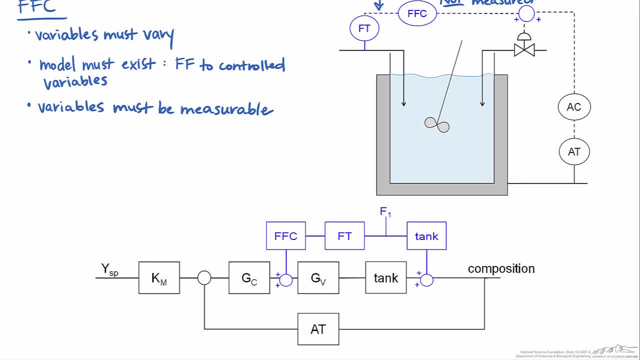 Now that we have developed our feedback and feed forward control scheme in a block diagram and therefore we can conduct a good amount of analysis, or put this into Simulink to kind of see how the processes act together. So to leave this, we'll have a few parting shots.